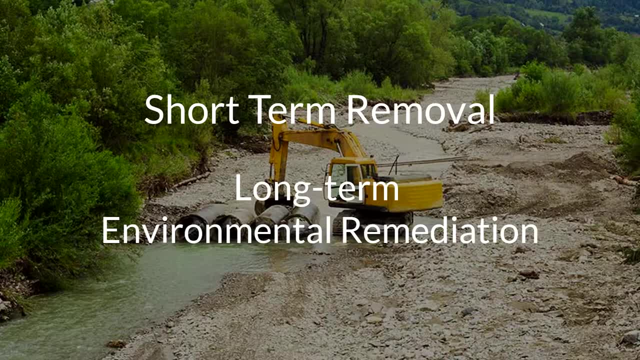 mitigate or, ideally, eliminate the threat. These actions deal not only with listed hazardous materials and substances, but also with any contaminants or pollutants, with the exception of oil and gas. The Environmental Protection Agency, the EPA, generally attempts to identify the responsible party for the mess, spillage or pollution that is being conducted only at sites listed on the EPA's National Priorities List, NPL. 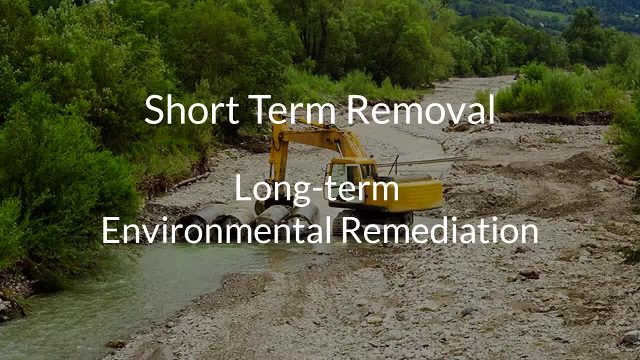 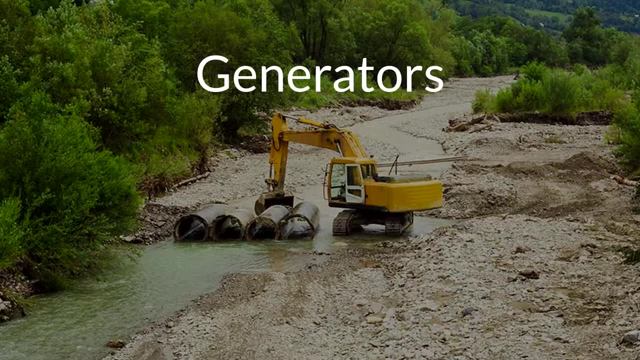 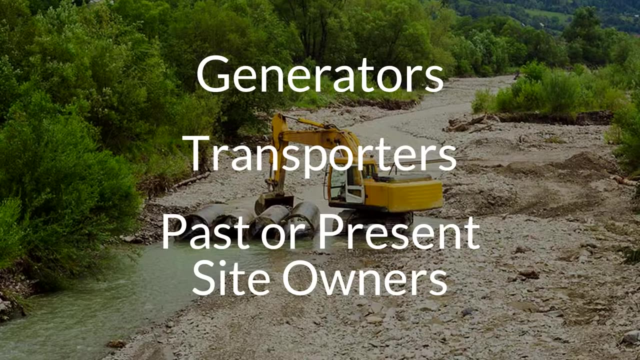 The responsible party for any contamination before taking response actions itself. Responsible parties can be any of the following: any generators of hazardous materials on location, transporters of hazardous materials to the site and past or present site owners. The responsible party has the option to willingly undertake the response task, but if they're unwilling, the EPA will order them to do it anyway. 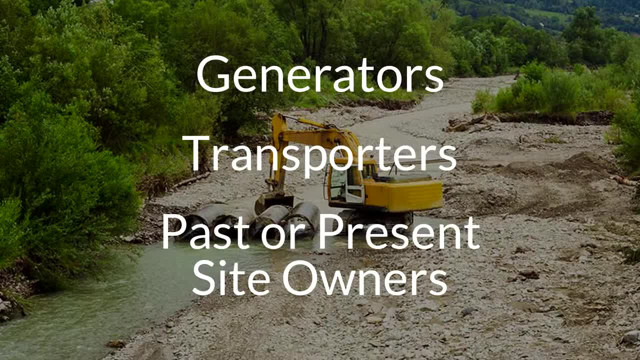 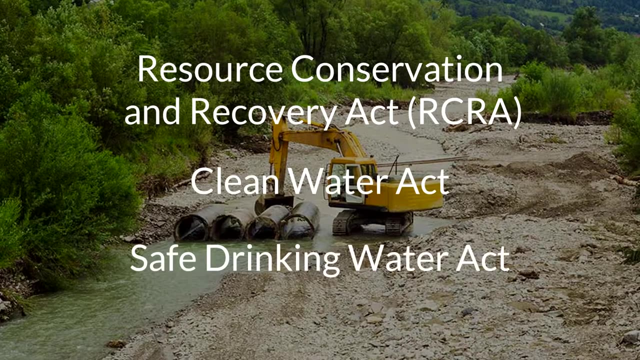 These actions are paid for by the EPA. These policies are paid for by the Ifil and can be offerd by a trusted fund made possible by a tax imposed on Chymical and Petroleum Industries. when CERCLA was enacted, CERCLA Powers and responsibilities overlap with the Resource Conservation and Recovery Act, the Clean Water Act and the Safe Drinking Water Act. 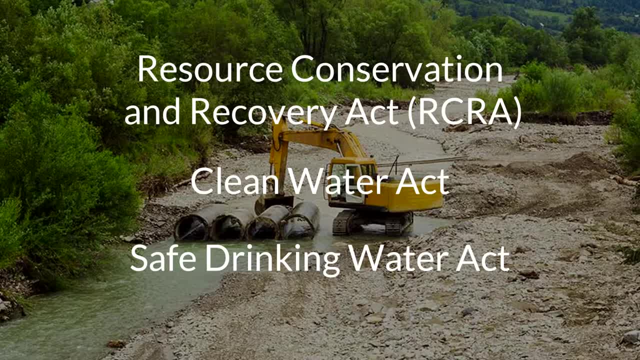 CERCLA and RECRA share jurisdiction with respect to hazardous materials and underground storageene是這樣 geography tanks containing petroleum products. guidelines for these tanks contained in Subtitle 1 of the 1984 Hazardous and Solid Waste Amendments to RCRA. However, the types of waste that are controlled are outlined by CERCLA. CERCLA was 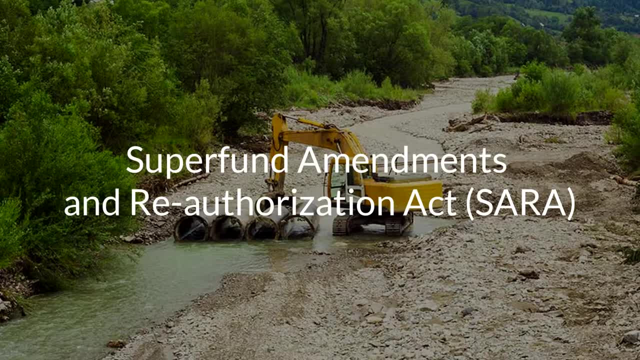 amended by the Superfund Amendments and Reauthorization Act SARA on October 17, 1986.. CERCLA is an important environmental program. It not only ensures that these invaluable removal actions are taken, but also enforces against potentially responsible parties and ultimately, 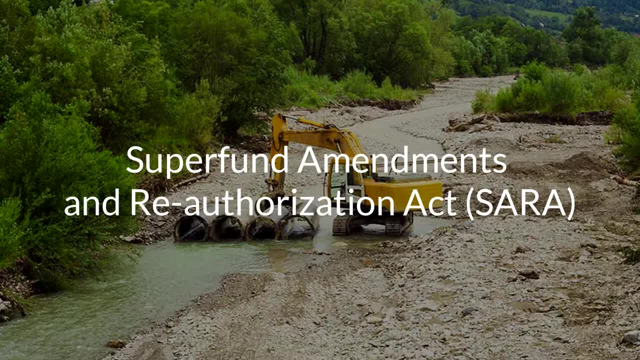 promotes strong accountability, community involvement and long-term protectiveness. One thing CERCLA cannot ensure, however, is perfection. Read our blog Trichloroethylene Concerns for Google employees to see why. Does your organization need environmental remediation services? If yes, we can help. 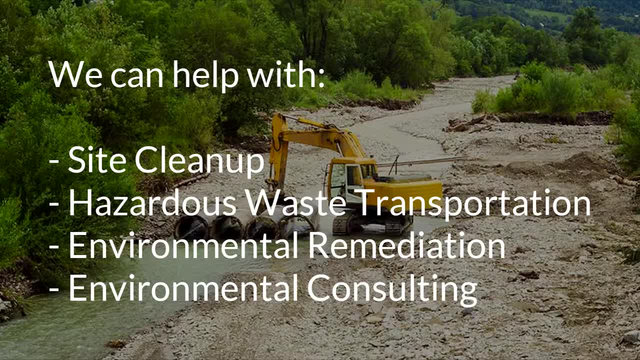 If your organization needs environmental remediation services, we can help. If your organization needs help with site cleanup, hazardous waste transportation and disposal, environmental remediation and environmental consulting services, call our experts at PEG-X or visit us online at PEG-Xcom. We offer our services nationwide.